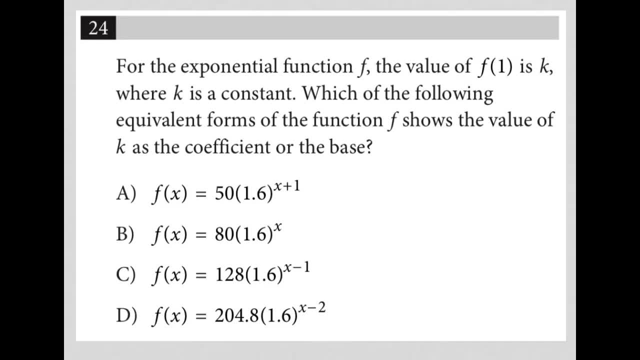 So this question says for the exponential function f, the value of f of 1 is k. I'll just write that down: f of 1 equals k. So I'm treating this like a translate word problem question where I want to write down any quantitative or any really relevant information from the passage. 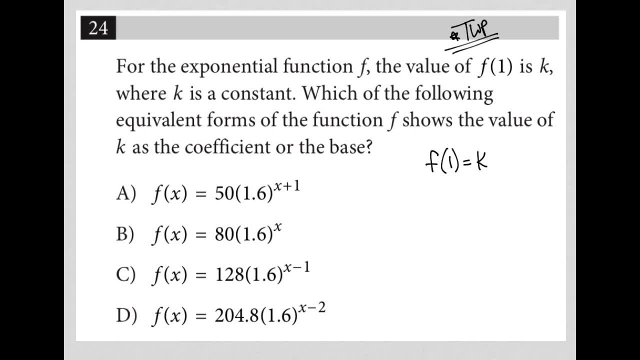 so that I don't have to go back and reread it later on. Which of the following: and k is a constant, right, so this is not a variable, it's a constant. according to the question, Which of the following equivalent forms of the function f shows the value of k as the coefficient or the 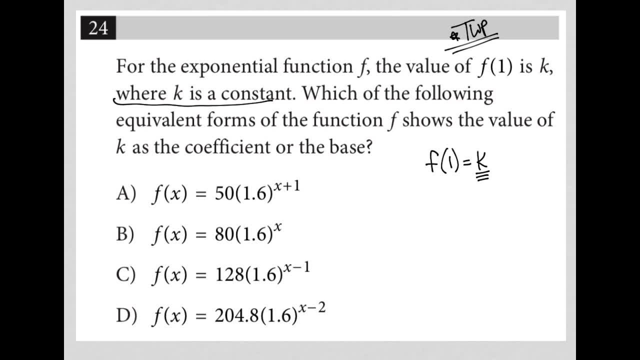 base. Okay, so what do I know? All I know is, when x equals 1 f of x, I'll say: when x equals 1 f of x is equal to k, Like this is literally what this means, right? I'm replacing the x with the k. So I'm replacing the x with the k. So I'm replacing the x with the k. So I'm. 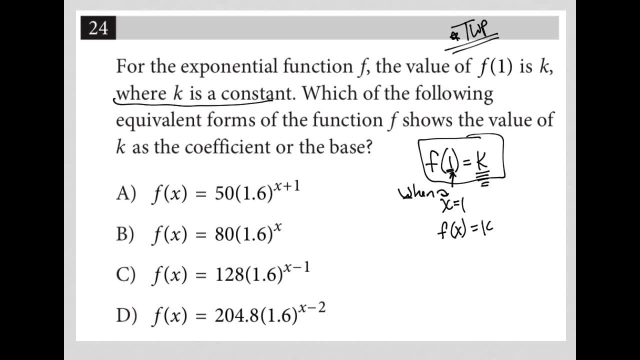 replacing the x with 1 and the answer I'm getting is a k. So I go to my answer choices now and I want to see: well, where can I get that scenario where I only get a single constant term on this side by plugging one in for my x value And that that k is a coefficient or a base, meaning that the 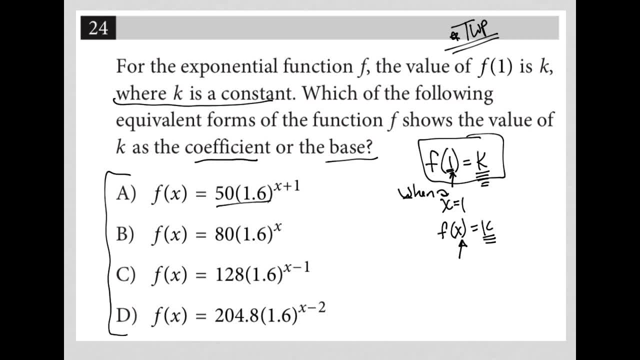 value that I get for f of x is listed here, So let me, let me go through these And then hopefully, if it's not clear, it'll help it make more sense as I go through it. So for choice a, if I replace x with 1, that makes this whole exponent equal to 2, and then I'd have 50. 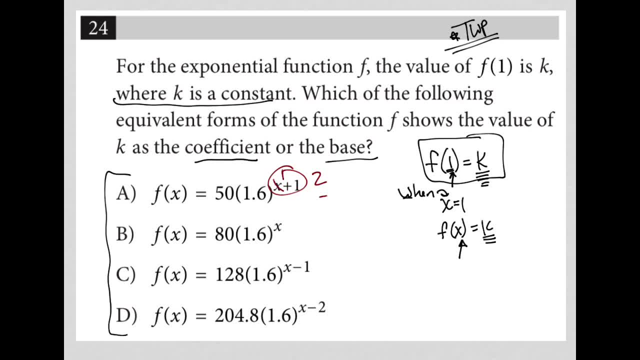 times 1.6 to the second power, which is going to give me some other answer. right, there's going to be some number that represents, and that number is not going to be here. right, it's not going to be. it's not going to be 50, it's not gonna be 1.6. that I get as an answer here, which means a. it's wrong.